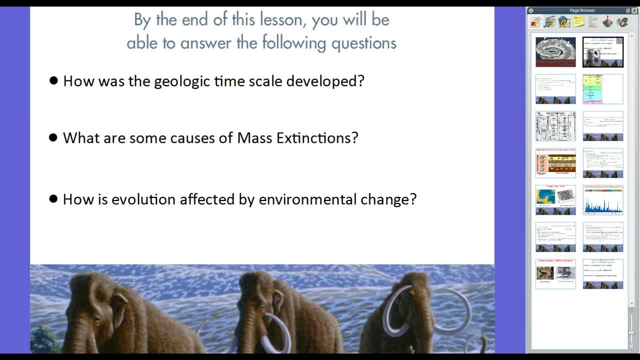 But first we're going to talk about how the time scale was developed, as well as pre-Cambrian time, before advanced life started really showing up on Earth. So anyway, by the end of this lesson, you'll be able to answer the following questions. Question number one was: how was the geologic time scale developed? Question number two: what are some causes of mass extinctions? And question number three: how is evolution affected by environmental change? So let's go ahead and dive into this. 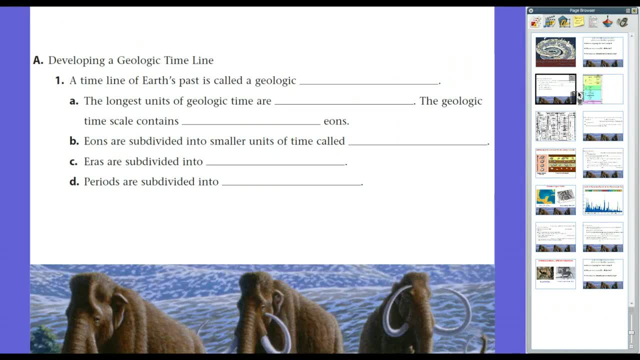 Just like in history, in social studies class, you have timelines. You know, on the left hand side of the page is the earliest event and as you go on and go forth you put important events and important times and things like that, until you get to the end of the event or present time. That's where you put all the far right. And scientists have that in terms, especially geologists, in terms of a geologic timeline. Okay, so geologists have constructed a history of the Earth and we put it all together in one big geologic timeline. Now there are four units of time in geologic timeline. 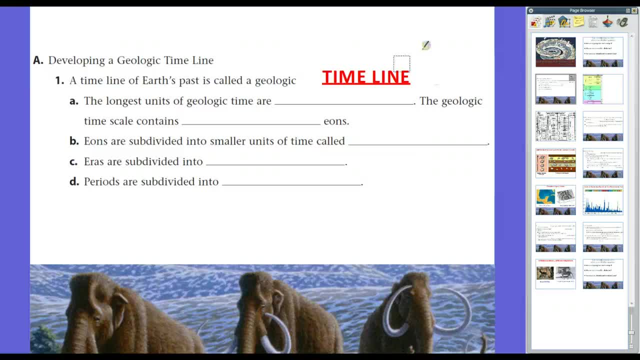 They go from big chunks of time all the way down to the smaller ones, And so the longest units of geologic time are what we call eons. The geologic time scale contains four eons which, when we look at the time scale, I'll show you them in a minute, but just for the record, they're the Hadean, the Archean, the Protos, the Pro-Arazoic and the Fan-Arazoic era. Okay, now eons themselves are subdivided into smaller units of time of what we call eras, And these eras are subdivided into periods, and these periods are subdivided into periods. 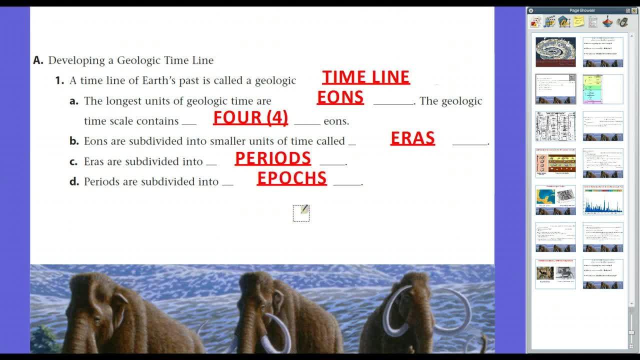 And these periods are subdivided into epochs, Yes, like it was epic, That's. it's a homophone, It's a word that sounds the same but has a different spelling and different meaning. Okay, think of it this way: in these four geologic time units, Think of eons as days, Okay, and days are divided into smaller units of time called hours, which would be kind of like the eras. Hours are divided into minutes, which are the periods, and the minutes are divided into seconds in terms of epochs. 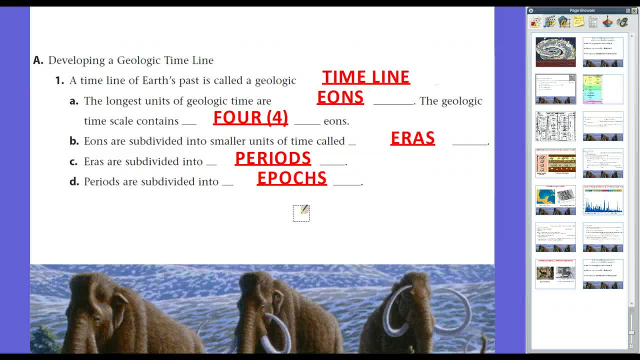 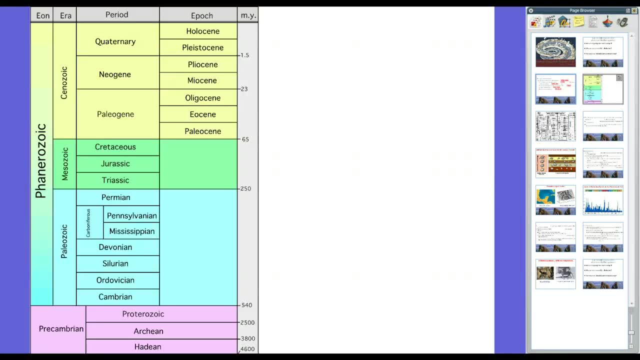 So eon, era period, epic, just like day, hour, minute, second. Okay, so there you go. So let's look at the geologic timeline. Okay, so here you go. Okay, so we have. we have Hadean, Archean, Proto-Arazoic and Fan-Arazoic era, and then this is divided into eras: Okay, the Paleozoic, Mesozoic, Cenozoic. Okay, these eras are divided into periods- Okay, Paleogene, Neogene, Quaternary, and divided into epochs. 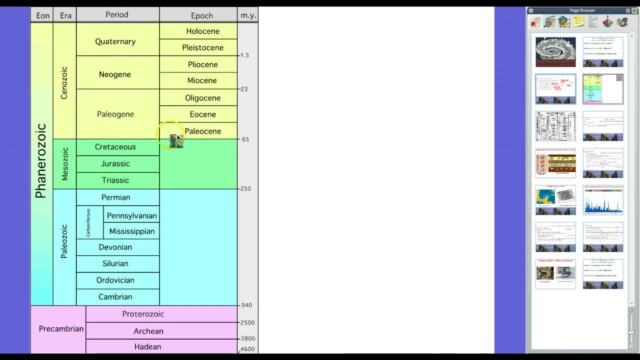 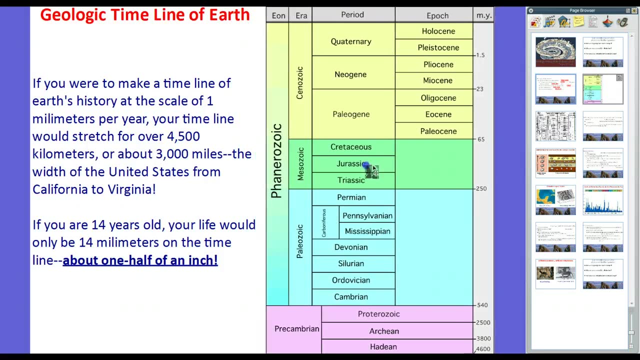 Okay, the Pleistocene Holocene. We live in the Holocene epic. Now, when we talk about the time, four and a half billion years- how long is it? It sounds like a lot, but how much is it? Well, if we look at the timeline like this and if we were to put this into a scale model where one millimeter would equivalent to one year, your timeline would stretch over 4,500 kilometers, which is about 3,000 miles. 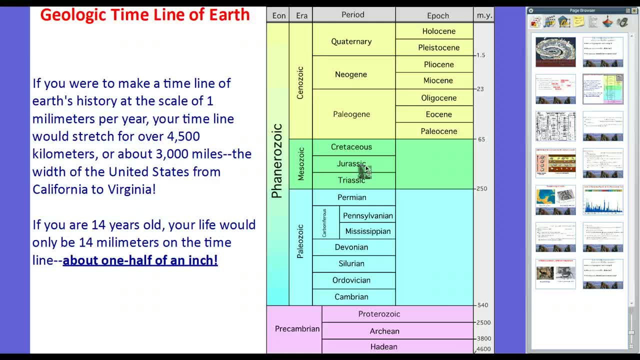 Essentially, the timeline of earth would stretch from California at the Pacific Ocean all the way to Virginia and the Atlantic Ocean. So essentially, the width of the United States would be the geologic timeline of earth. Okay, that sounds pretty big. Now, how do our lives fit in? Well, think about this: If you're an eighth grader, you're either 13 or 14 years old. Okay, so based on the same scale, your life would be 14 millimeters in length, so 1.4 centimeters. 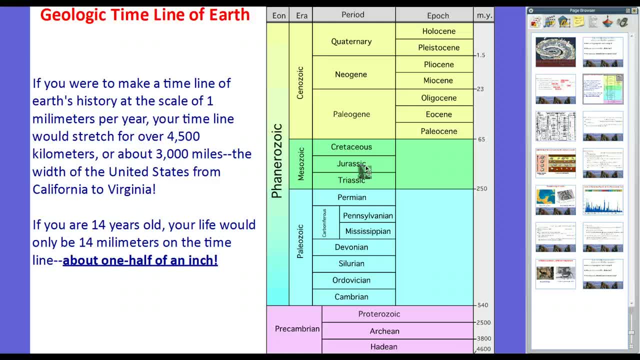 okay, how long is? 1.4 centimeters? about one half of an inch. so how much of your life is? in comparison to the entire history of the earth based on our dating methods, apparently not very much at all. one half of an inch is comparison to the entire width of the united states. that's pretty small. 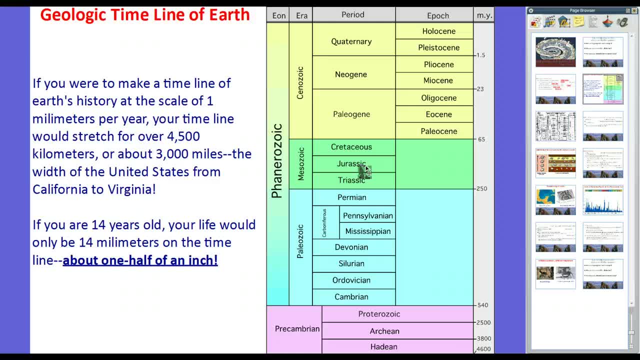 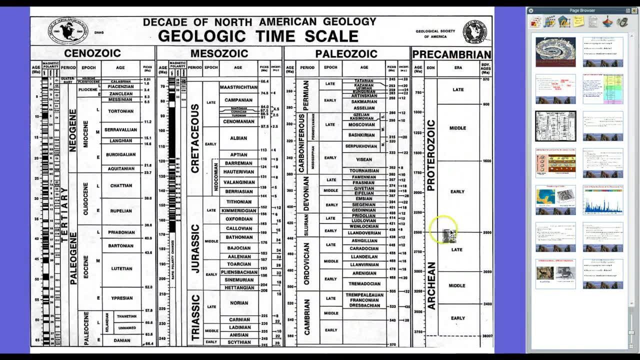 pretty insignificant. now, of course, we can go into even further detail, as this completely complicated looking geologic time scale. we have pre-cambrian time, okay, and then see, we have, we have age, we have, let's say, we have the period, we have the epic, these are the eras. 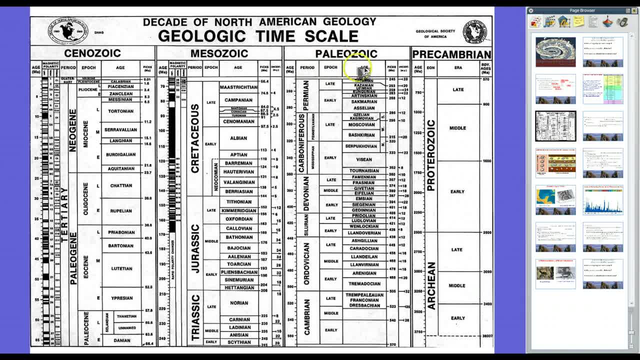 okay, uh, period, epic age, and then the timelines of them themselves, and even right here about magnetic polarity based on the magnetic pulse flipping this from the, uh, north american geologic geological society of america during their decade of north american geological anyway. so, needless to say, we can divide time up into really small times, okay. so how were we able? 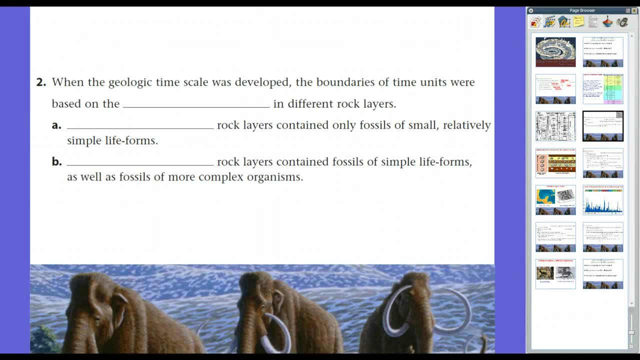 to figure this out. well, mainly we began piecing it together based on the fossils in different rock layers. so essentially the geologic time scale was kind of put together by relative age dating. we knew that the further down you go, the older the rocks are, and only through radiometric dating were able. 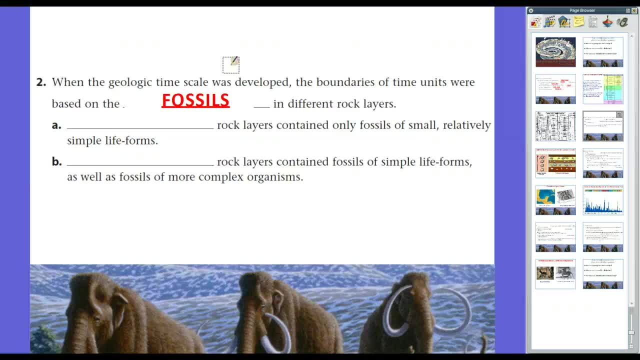 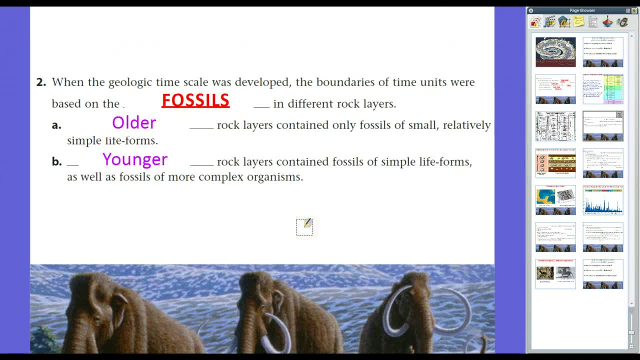 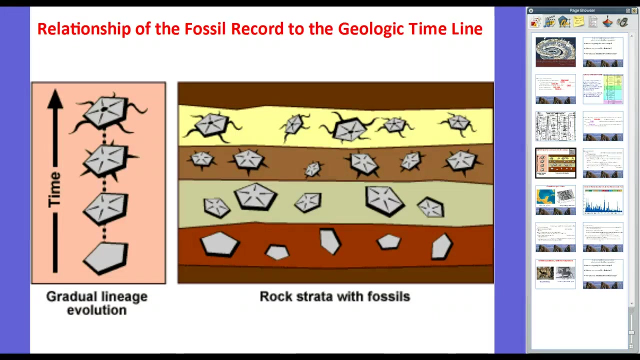 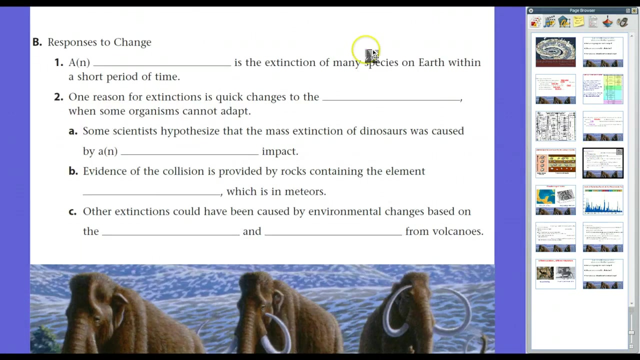 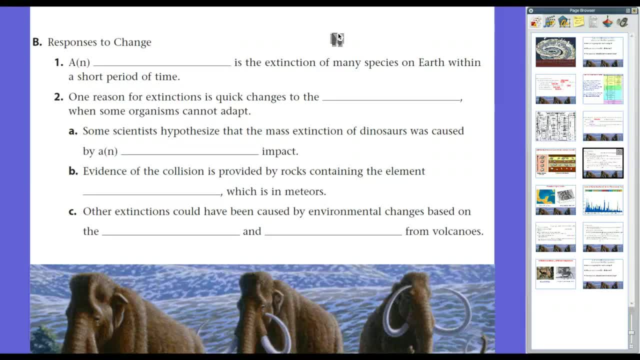 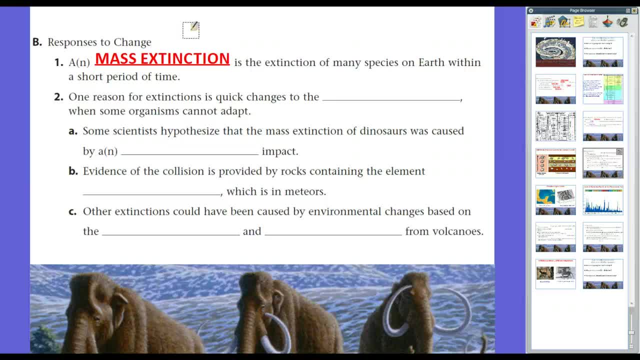 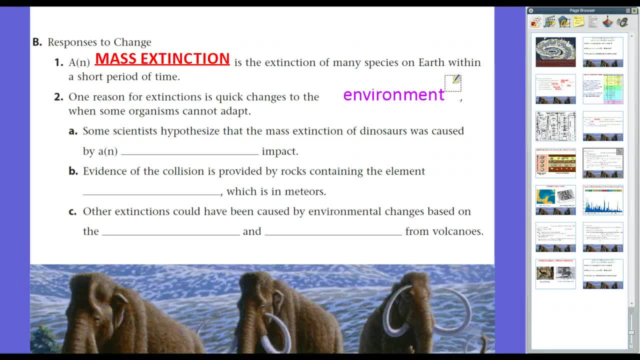 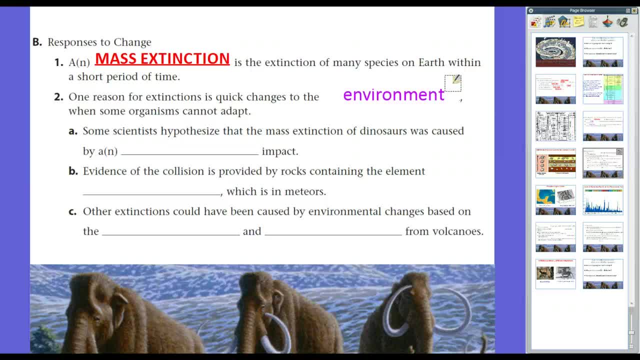 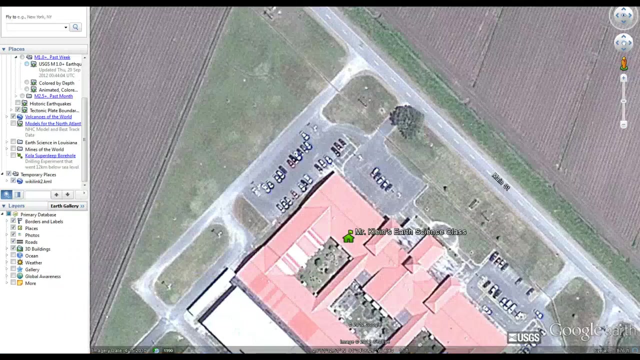 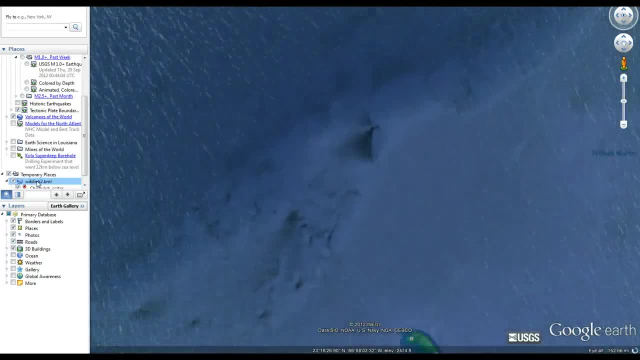 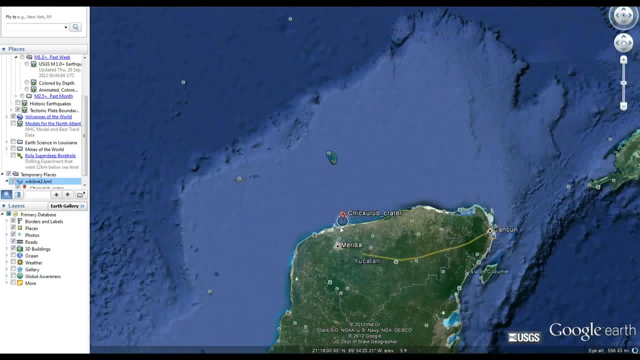 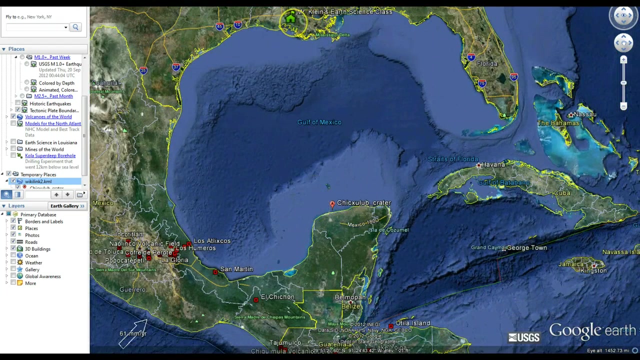 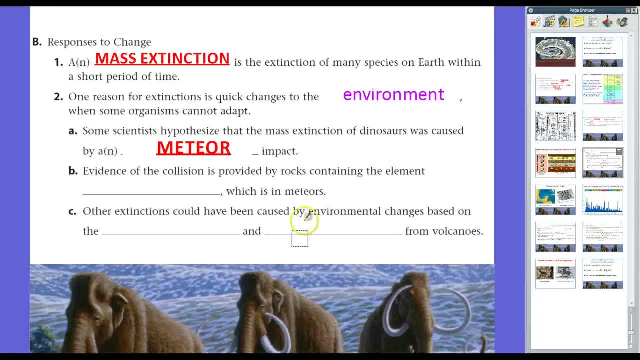 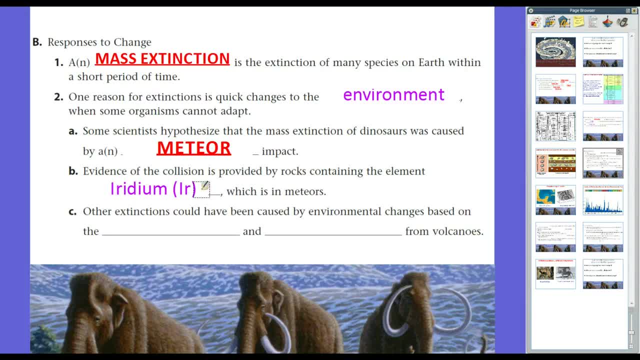 which is really rare on Earth, but in meteors it's full of it, And what they have what's called is the K-P-G line in the rock layers, And there's a very thin layer that divides the Mesozoic era with the more recent era, the Hologene era. 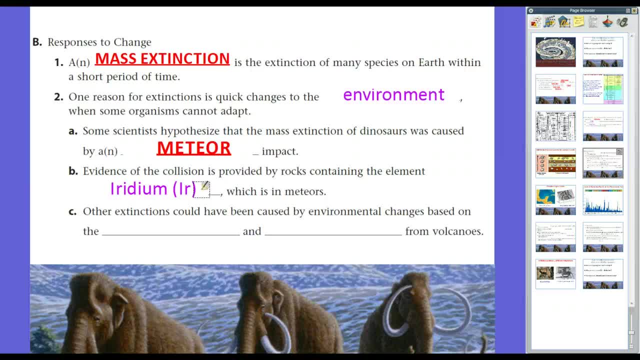 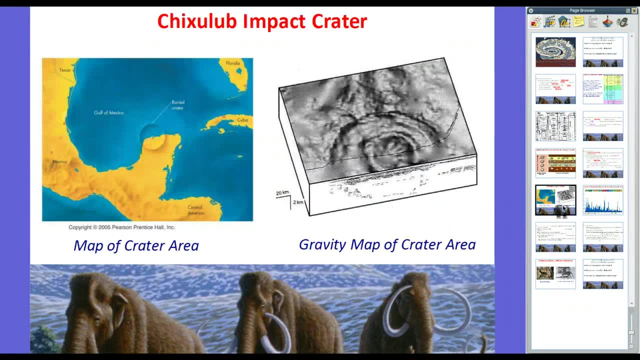 And essentially in that thin layer of rock, which means it was really short on the geologic timeline- there's a lot of iridium in it, And so let's look at the Chicxulub Crater. The buried crater is about this size in the Yucatan Peninsula, like I showed you. 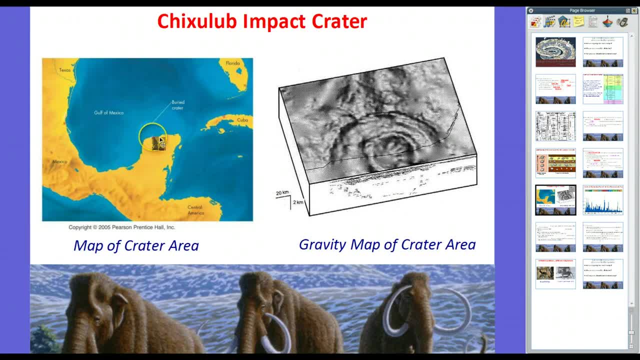 So it's pretty big And here's the exact impact, which is just off the coast, And since it was 65 million years ago, a lot of rock has covered it over. However, evidence of rocks pulled up in boring and drilling for oil. 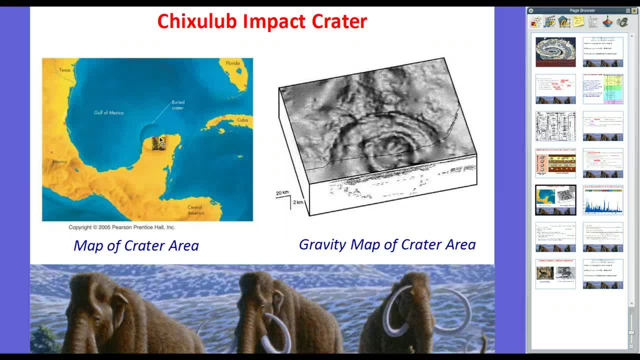 showed that it looked like there was some sort of impact, and scientists began studying, and studying, and studying. And, for example, what you have on the right right here is a gravity map. It shows the layers of gravity And, as you can see, here's the coast of the Yucatan. 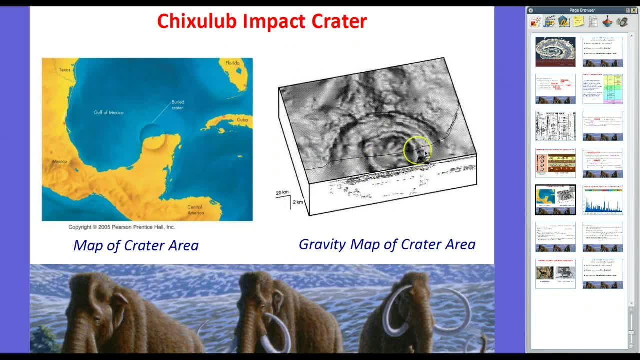 And it's this right here. And what do you notice? A giant hole in the ground going down over 2 kilometers and about 20 kilometers across. So that's a huge hole. That's what: 12,, 13 miles across, over 3 miles deep. 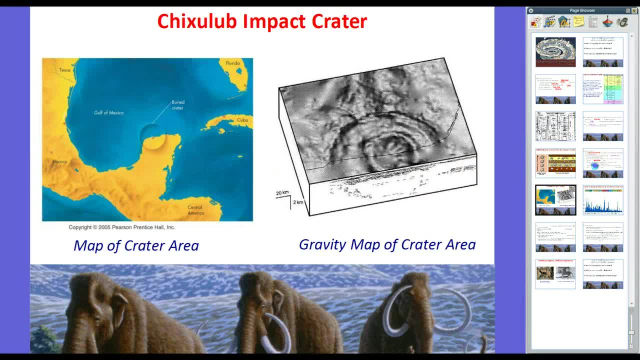 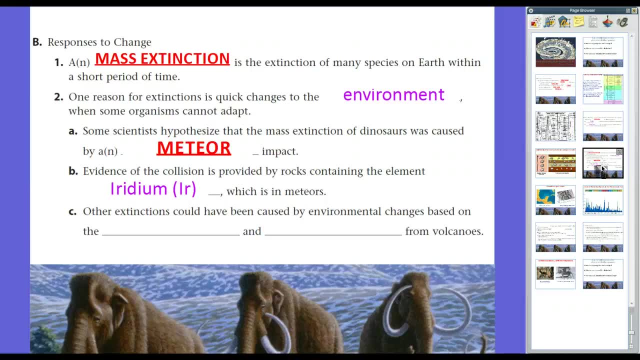 Okay, is the size of the crater. So that big of a crater, throwing out that much dust and stuff, would have caused massive global climate change which would have killed off tens of hundreds and thousands of different species. okay, causing radical changes on there. 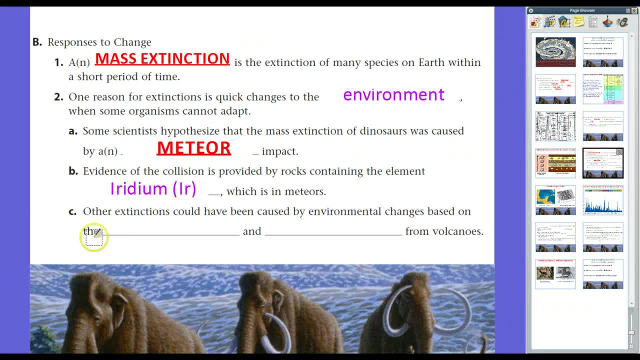 Now in the past, which we'll look at, other extinction events. they could have been caused based on the gas and dust being released from massive volcanic eruptions And, in fact, the biggest extinction event of all time, which is right here. 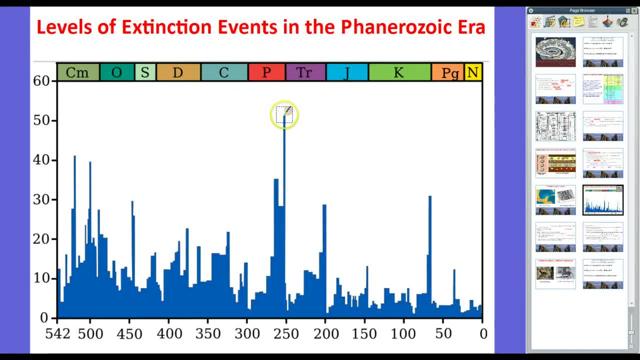 at the end of the Permian and the Triassic era right here, pretty much about 96% of all marine life, in other words, all ocean-going organisms, died And over 70% of land-based organisms died in the Permian-Triassic event. okay, 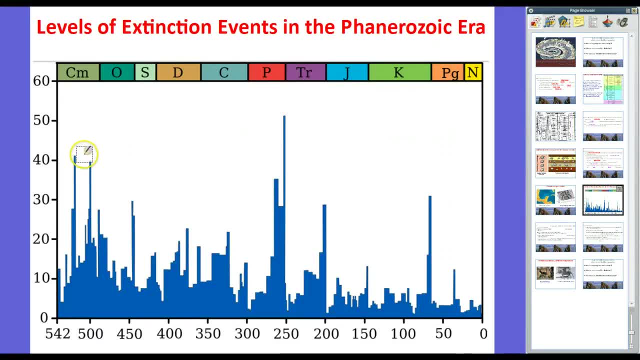 So that's the biggest extinction event, And then here's some other ones in the Cambrian time, in Ordovician time, right here, probably caused by meteorites, a meteor strike here, But right here it's hypothesized that the Permian-Triassic event. 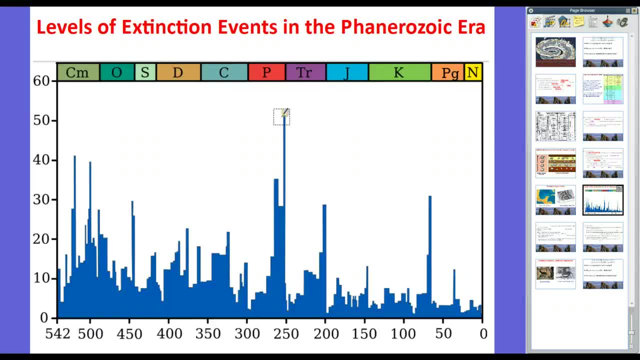 might have been caused by massive volcanic eruptions all over the world, And so much gas and so much dust was pumped into the environment that the climate changed radically and that's why you had so much death And, as you can see right here, 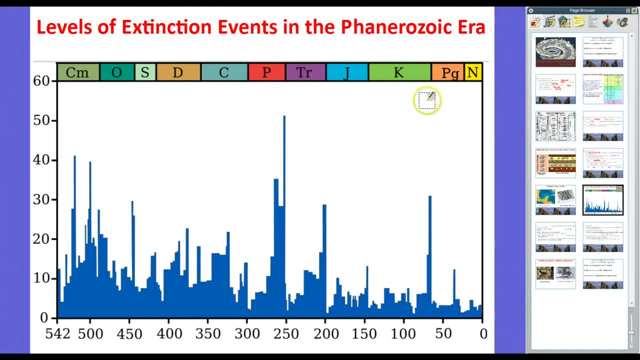 about 65 million years ago is the end of the Cretaceous period, which is the end of the Mesozoic era and the beginning of the Paleogenic era. okay, Okay, So I'm sorry. the Paleogenic period. 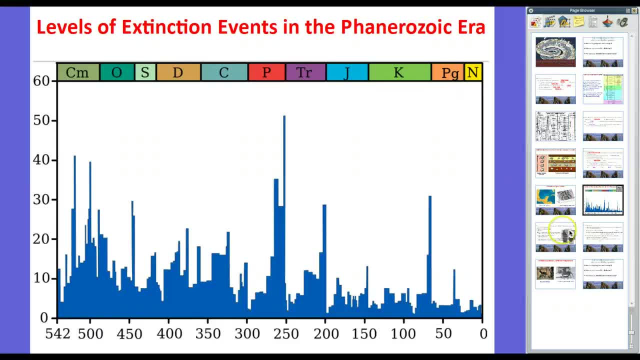 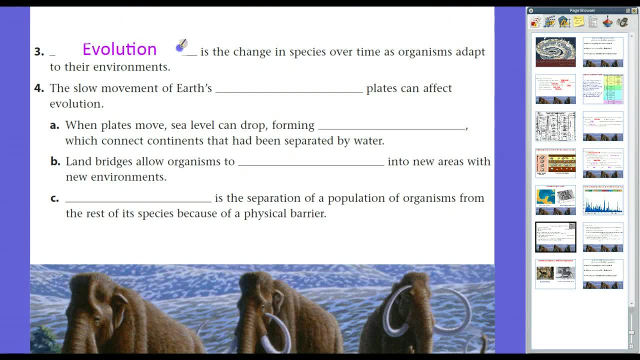 So there you go. That's levels of extinction events. okay, going on throughout time. Now going back to last year and talking about natural selection, we know that evolution is the change in species over time as organisms adapt to their environments. 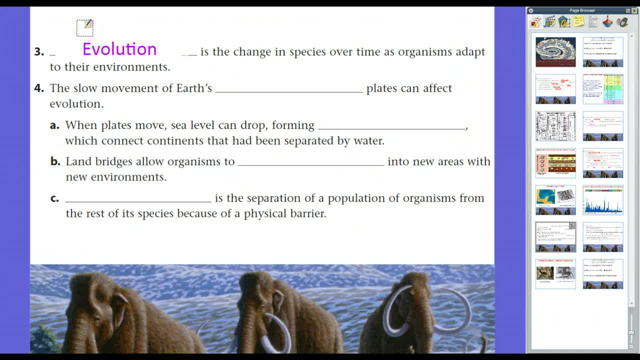 Natural selection states that the organisms which are best suited to survive will be the ones who can adapt the best. Now, in addition to this, the slow movement of Earth's tectonic plates can affect evolution too, So it's not just mass. 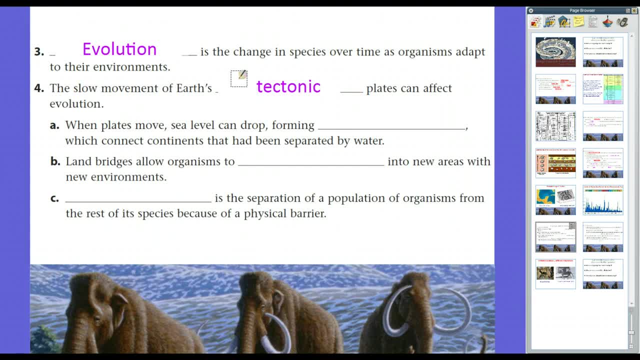 Massive. you know catastrophes that cause this. It's not catastrophism but also uniformitarianism. The geologic forces are taking place at slow rates. For example, when tectonic plates move, sea levels can drop, forming land bridges. 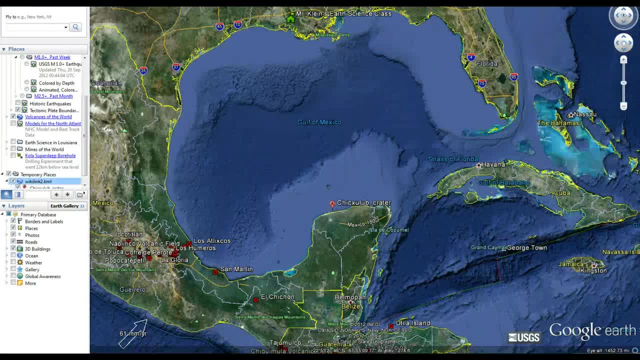 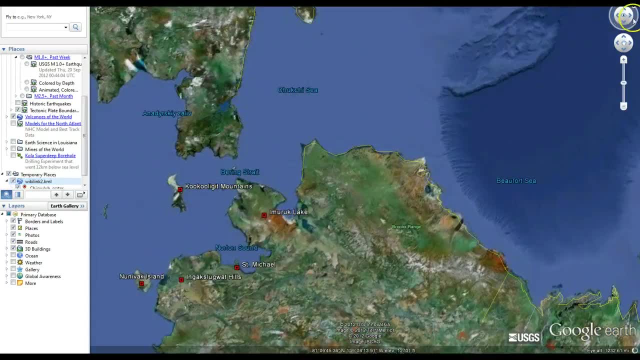 which connect continents that have been separated by water, And the most famous land bridge we're talking about, if we zoom out of Earth, okay, and we go and we look right, here is what we call the Bering Land Bridge And the Bering Strait. okay, 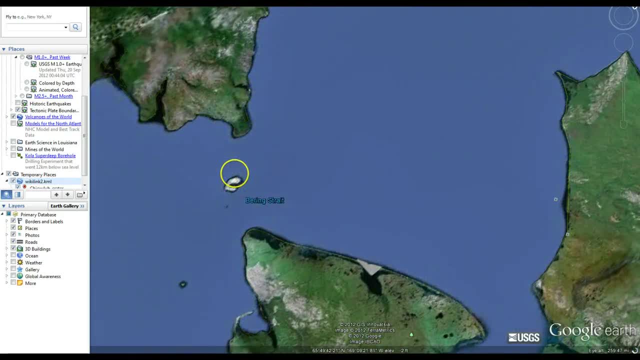 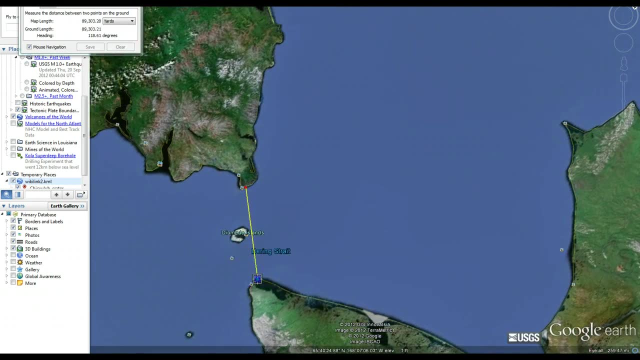 connects Russia and the Bering Strait. okay, connects Russia and the Bering Strait. okay, connects Russia and Alaska. And this is really really close. okay, Just for the instance, from here to here is only 81 kilometers, or 50 miles. 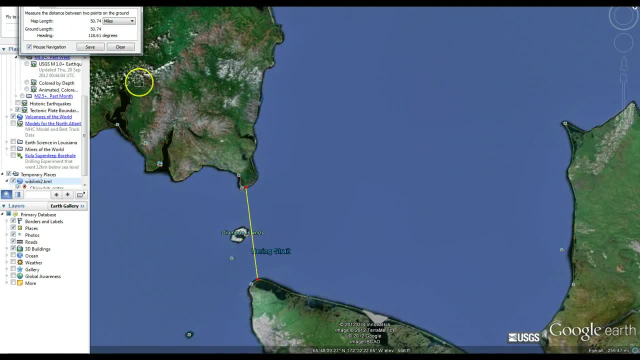 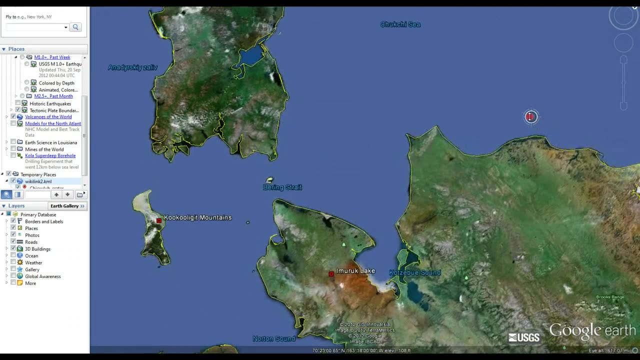 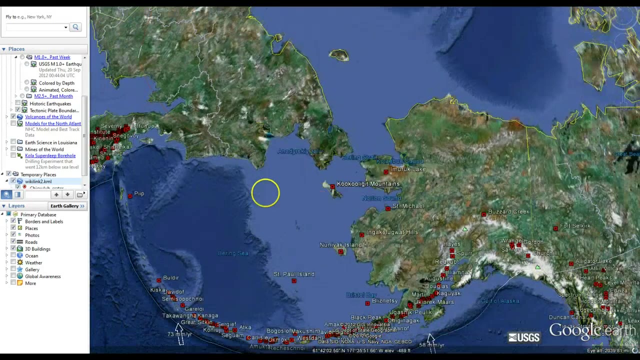 So Russia and Alaska are only separated by about 50 miles And during previous eras of geologic time, this area, this area, was actually connected by a land bridge because, as you can see, the continental shelf, which is this really just really shallow area. 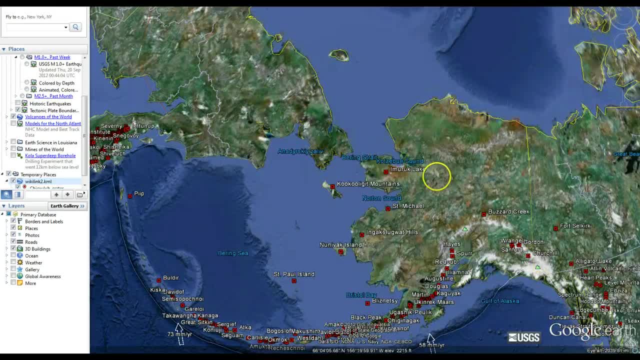 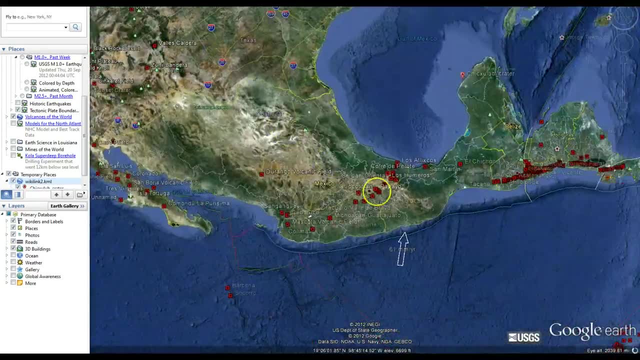 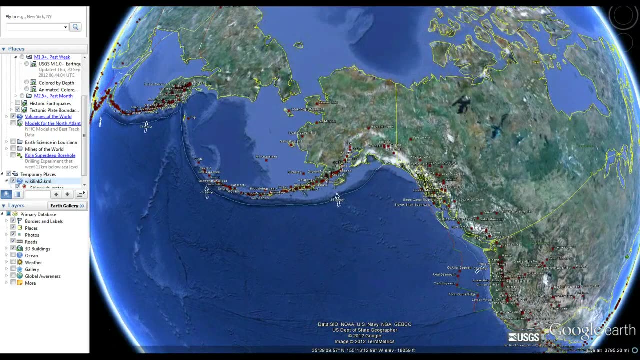 the sea levels went down and this was exposed land. So in other words, Asia and North America were connected And organisms and even people migrated across and they came down here and they eventually settled all of North and South America. Okay, so the Bering Land Bridge is an important 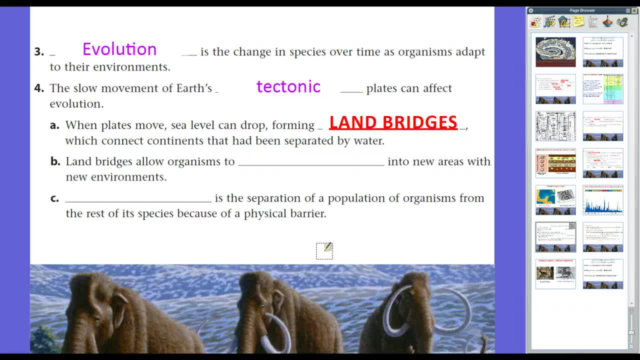 important concept in evolution, because organisms were able to transfer from one way to the other. Because whenever we look at the Cenozoic Era and we look at Ice Age and stuff like that, that you had mammoths like seen right here. 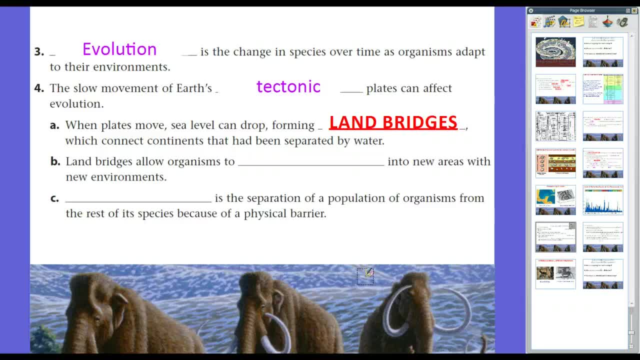 or mastodons in addition, or saber-toothed cats, or dire wolves, or lions or bears, and all these that look just like their old world counterparts that you might see in Asia or Africa, but they were around in North America. 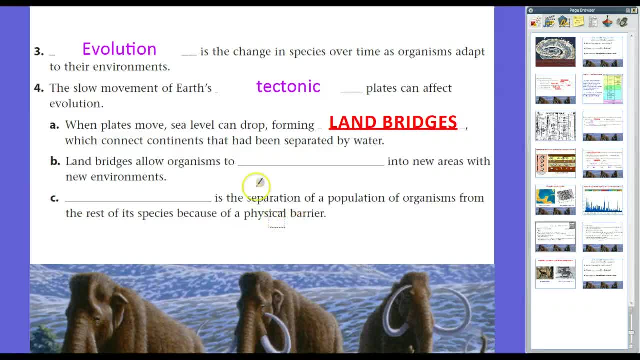 And eventually, And eventually, climate change and stuff happened and they all died off. So, like I just said, land bridges allow organisms to move into new areas with new environments and then they would have to adapt to them. Now, the term geographic isolation: 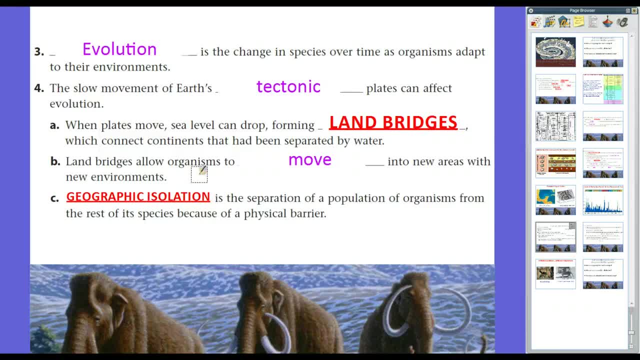 is the separation of a populism of organisms from the rest of its species because of a physical barrier. So, for example, climate change happens, sea levels go up, lions are separated. okay, There are North American lions and then there were European Asian lions. 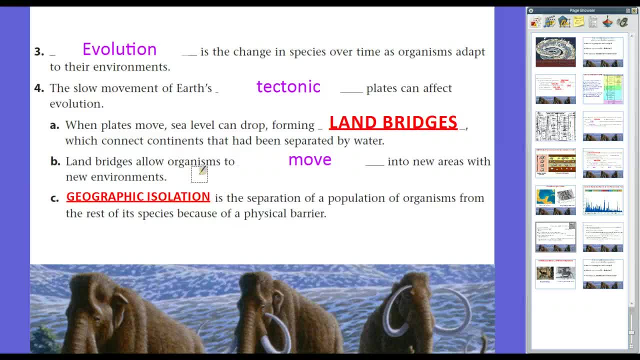 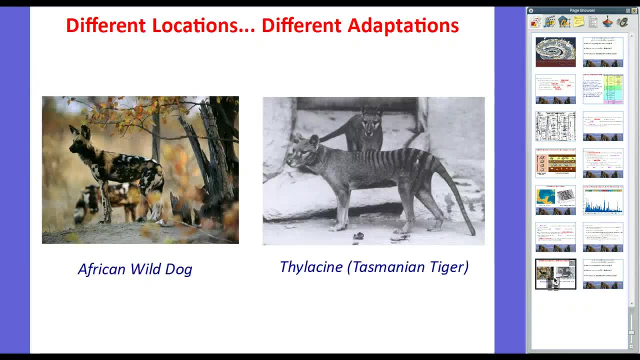 and stuff like that. okay, So those were separated and as a result of their separation, over time, they'll evolve differently. Now, according to the theory of evolution, that you have common ancestors, okay, That's one theory, And another theory is that, even that when organisms 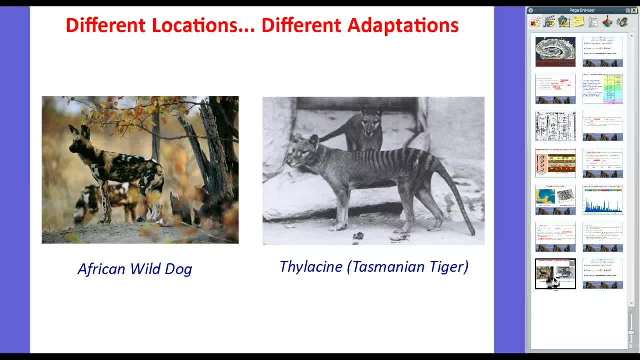 go into different biomes. they adapt and fill in certain ecological niches or certain ecological roles. Take, for instance, the African wild dog and the thylacine, or the Tasmanian tiger. okay, These are actually not related at all, okay. 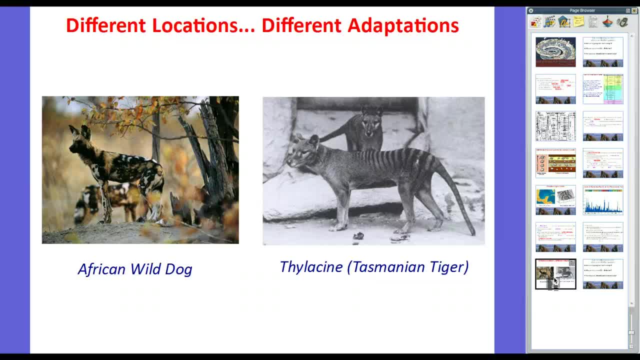 Wild dog is a canine not quite related to dogs, but it's a distant relative. The thylacine, however, is most closely related to a kangaroo. Now, if we go back in the evolutionary tree far enough, they will have a common mammalian or a mammal ancestor. okay, 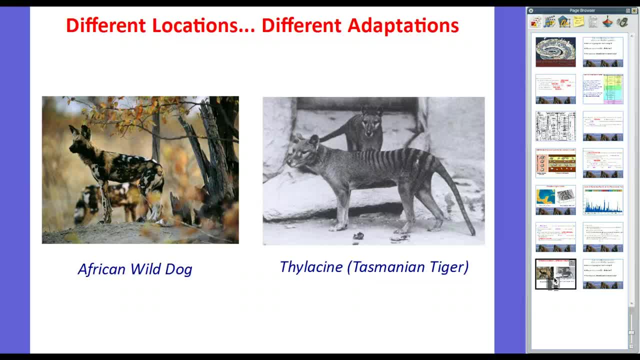 But the African wild dog, of course, is in Africa, The thylacine was in Australia, And because they had similar ecological niches, if you look at their bodies and look at their shapes, what do you notice about them? 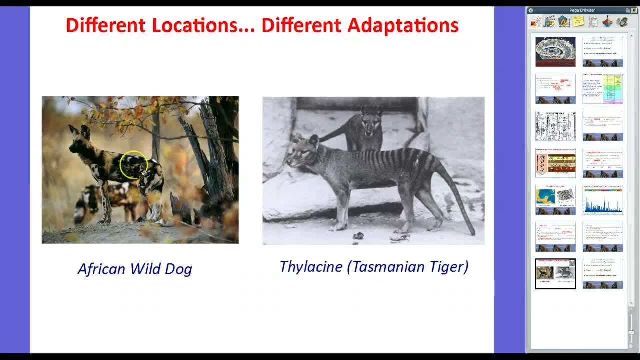 They have broadly similar features, You notice. their faces are kind of the same And they were both predators and they preyed on small animals. okay, And the thylacine sometimes ran in packs, sometimes they ran individually. African wild dogs have pack mentality. 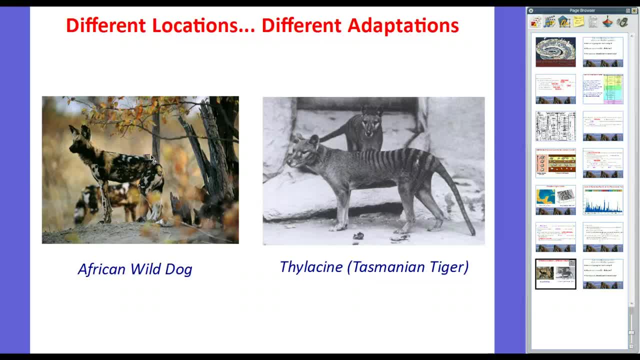 and they don't operate alone, okay. So, because of geographic isolation, Australia was way off from everywhere else. You had a lot of different adaptations and because Australia views were all different and they were all the same- okay, Because those differentÓ. 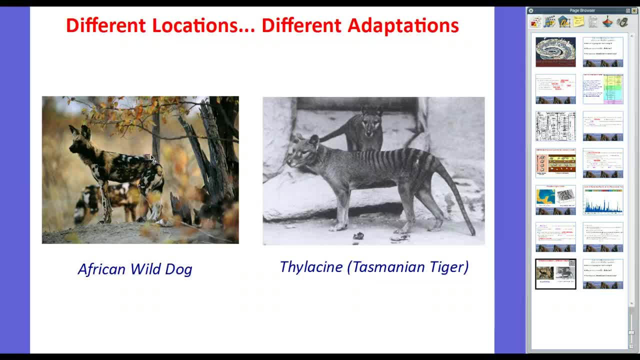 Okay. so because of geographic isolation, Australia was way off from everywhere else. was uh moved off, uh isolated long ago. the common ancestor, where it breaks off, allowed for radically different evolutionary uh changes take place. so that's why you have a thylacine, as compared to 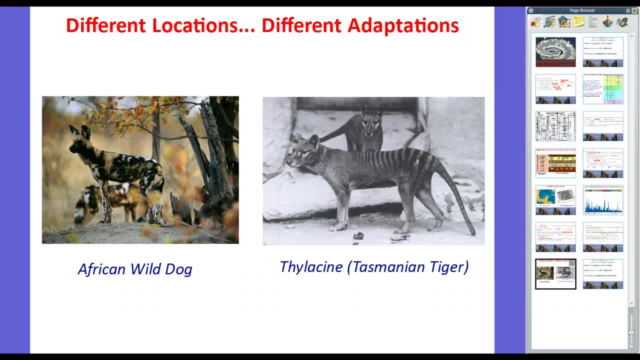 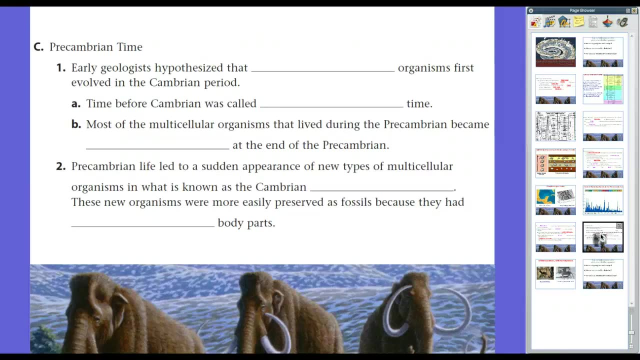 wild dogs. in fact, dogs weren't even on australia until, um, until people started showing up, and then you ended up having the dingo. okay, so there's your lesson, okay? geologic history of the earth: uh, which will wrap up right here with the beginning of the beginning of time of organisms. 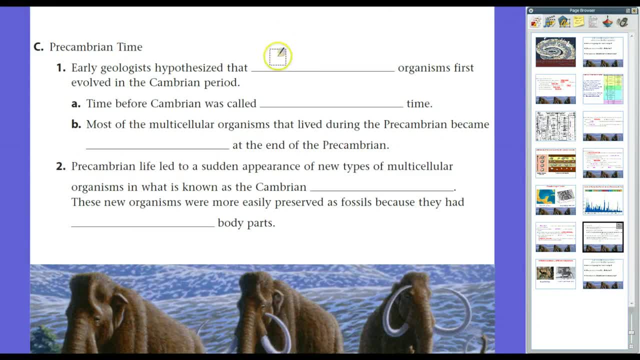 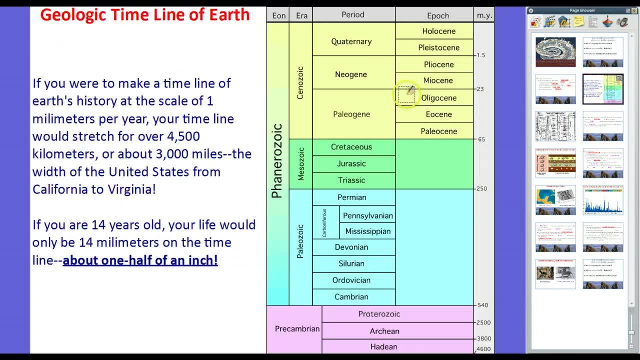 and essentially pre-cambrian time. in pre-cambrian time, early geologists- uh hypothesized that multicellular organisms first evolved in the cambrian period, which will bounce up right here: okay, the cambrian period is only about 540 million years ago. okay, so that's usually when we think of. 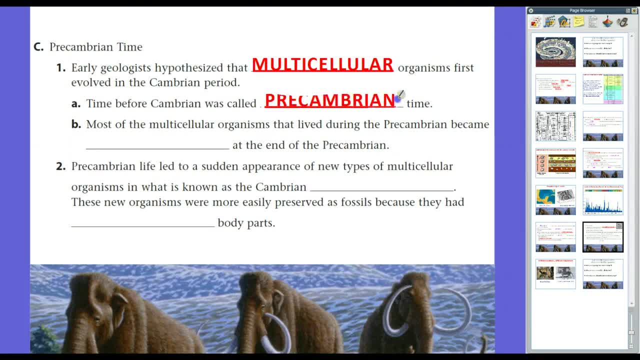 when life starts kick-starting now. time before came period time before Introvertism came about 540 million years ago. okay, so that's usually when we think of when life starts kick-starting now. time before cambrian. cambrian was what we call pre-cambrian time. okay, so essentially, from four billion four and a half. 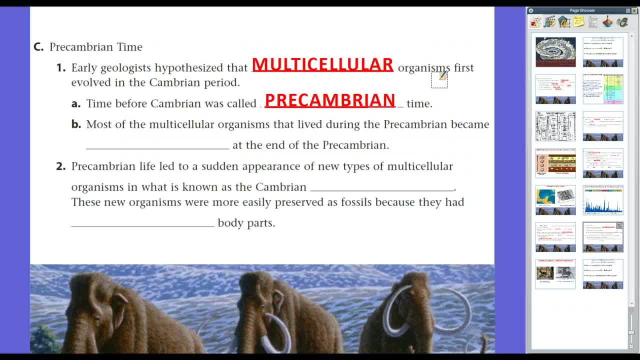 billion years ago, up until 540 million years ago, there's essentially life. if it wasn't here, it was only in, you know, cellular, single-celled organisms. we call that pre-cambrian time. that's when a lot of meteors happen. you know, uh, a mars size planetoid skimmed off of earth probably formed the moon. 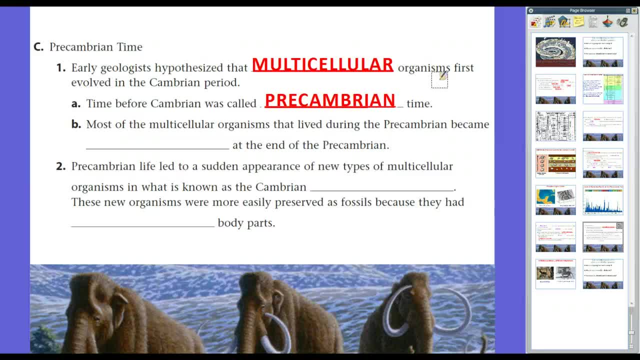 things like that. when we talk about the formation of solar system, we'll get into that, okay. so a lot of major geologic changes were taking place and most of the multicellular organisms that lived during the pre-cambrian became extinct at the end of the pre-cambrian period. okay, climate change. 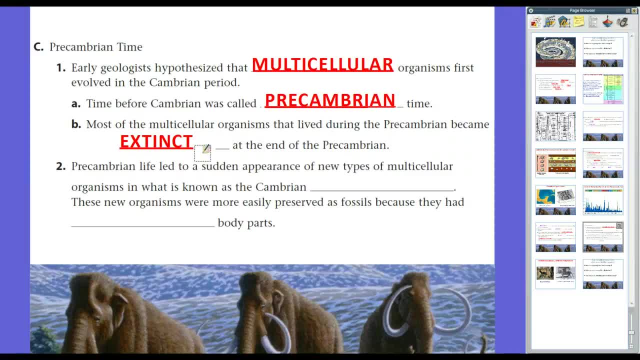 meteor impacts, stuff like that, caused that. however, pre-cambrian life led to a sudden appearance of new types of multicellular organisms and what we know as the cambrian explosion. essentially what happened is, if we look at the fossil record, we just have little multicellular organisms, little. 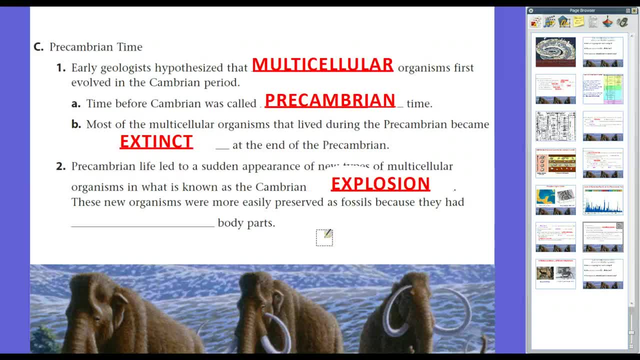 plants, proto plants, things like that. all of a sudden, 540 million years ago, bang okay, uh, everywhere life, everywhere, in all sorts- plants, invertebrates, animals. all that was the cambrian explosion. and these new organisms are more easily preserved as fossils because they had hard body parts, like 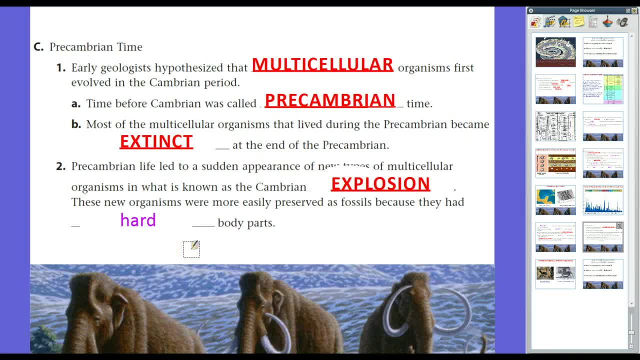 for example, you remember the trilobite at the museum? that's that little crab looking thing. okay, they had a hard exoskeleton, which means when they were buried quickly during pastures and things like that, they were able for them to be fossilized. okay, so in terms of the 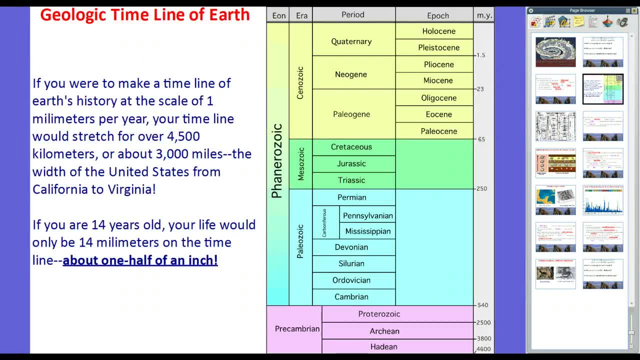 geologic timeline we've covered. we covered about 4 billion years. pre-cambrian time only makes up about 4 billion years. okay, and so what we did is we started talking about the cambrian explosion and we're going to move through here over each lessons, especially sitting on the paleozoic. we're 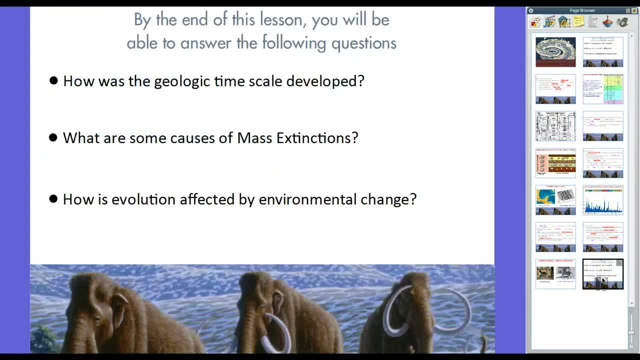 going to sit on the mesozoic and we'll go on the cenozoic, okay, so let's wrap up this lesson. uh, so how was the geologic time scale developed? well, scientists developed the geologic time scale through the relative age dating of rocks, as well as the examination of fossil record. what we saw was: 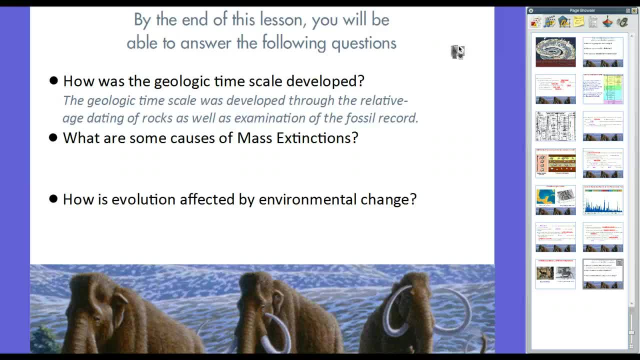 the older the rocks were in the geologic column, the more simple the organisms, and so, putting two and two together, we figured that as life evolves on planet as time went on, and only through absolute age dating methods, we're actually able to pin down the ages of these rocks. now, what are some causes? 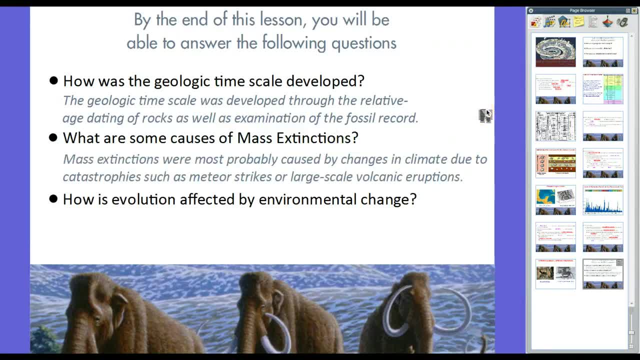 well. mass extinctions were most probably caused by changes in climate due to catastrophes such as meteor strikes or large-scale volcanic eruptions. huge meteor hits the earth, creates a huge crater, causes huge global climate change, lots of things die off- or large-scale volcanic eruptions, which